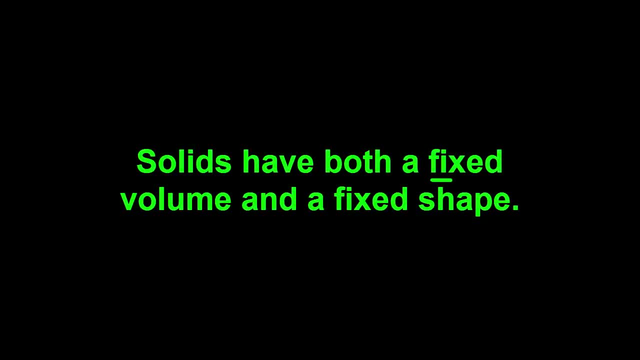 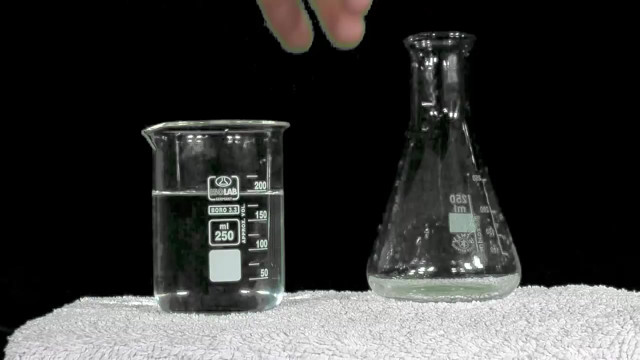 Solids have both a fixed volume and a fixed shape. Their fixed volume and shape means that solids are rigid. Can we change the volume of a liquid? Here's a beaker with a volume of 200 millilitres of water in it. 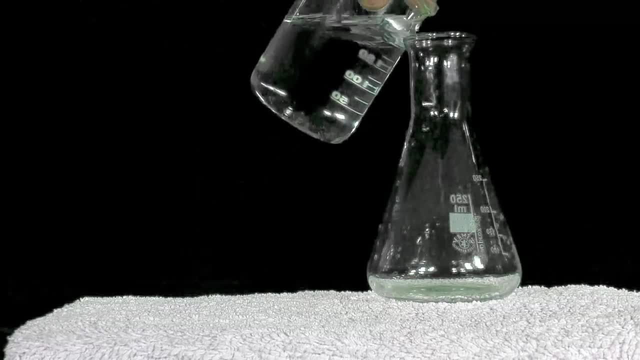 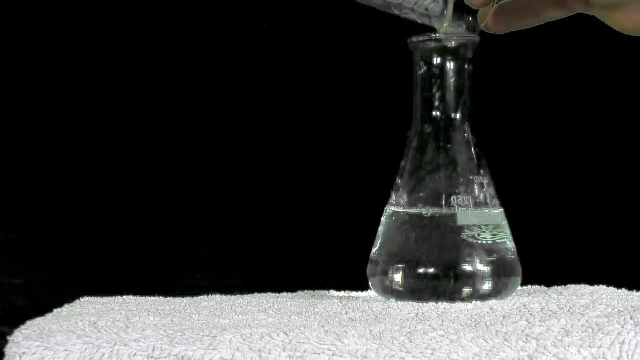 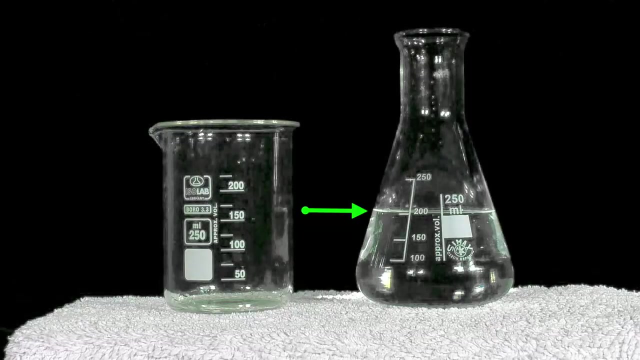 Here's a beaker with a volume of 200 millilitres of water in it. Has the volume become larger or smaller when we pour it into a flask? Trick question: It's still 200 millilitres, so it's volume hasn't changed. 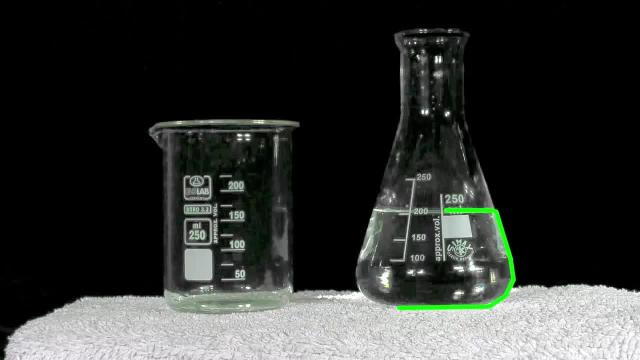 How about its shape? In the flask, the water is the shape of a cone, Same as the shape of a flask. When we pour the water back in the beaker, the volume of the liquid is the same as the shape of the flask. 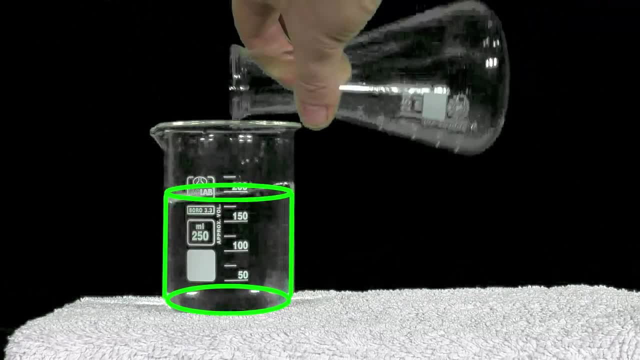 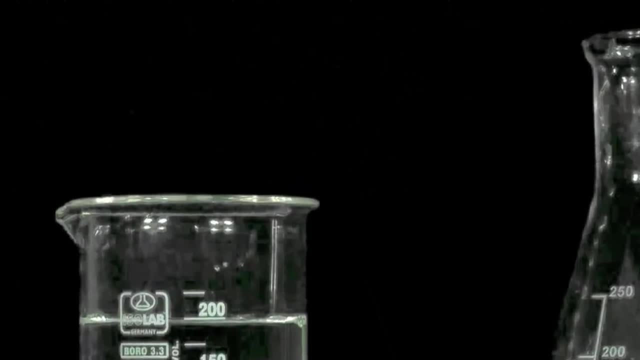 But back into the beaker, its shape becomes cylindrical, same as the beaker's. The shape of a liquid changes to match the shape of the container it's in. This means that liquids have a fixed volume but a changeable shape. 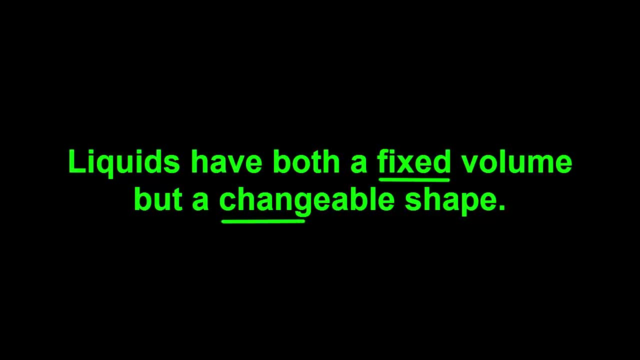 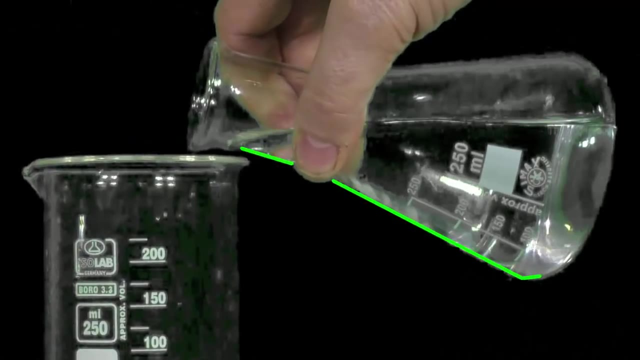 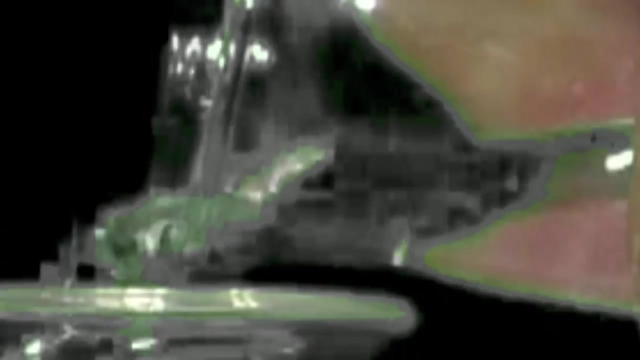 Music. Water's weight and changeable shape makes it find the lowest place in its container. As the water reaches the lip of the flask, there's nothing to hold it back and its weight pulls it outside the flask and downwards in a stream. Music. 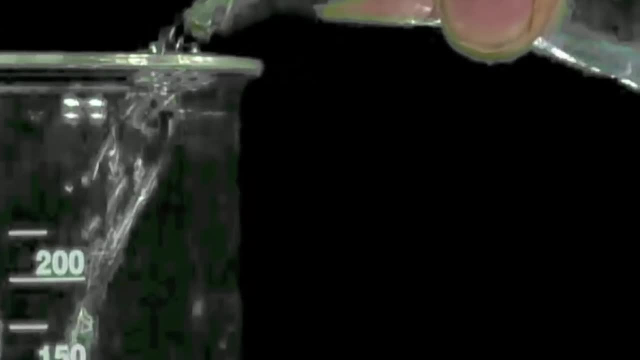 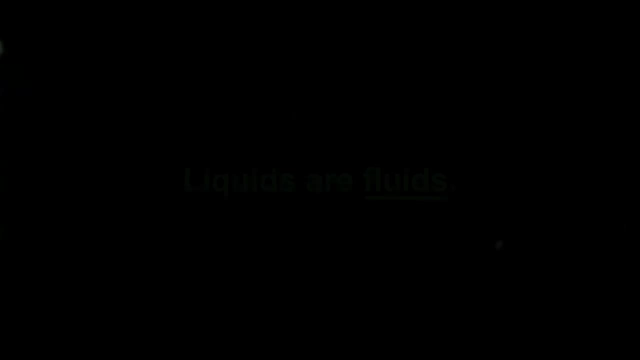 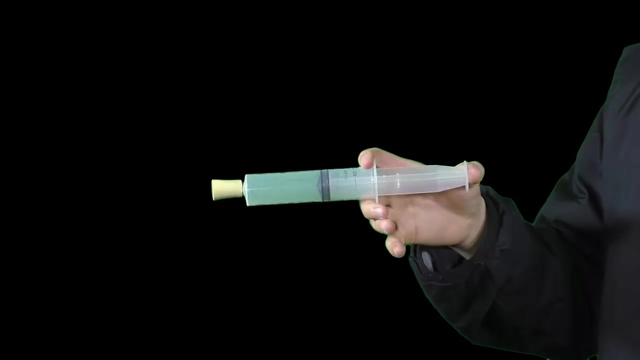 Water's changeable shape enables it to flow Music. That's why liquids are called fluids Music. Can we change the volume of a gas You bet? Here's a syringe with 50 millilitres of air inside and sealed at its tip so that it can't escape. 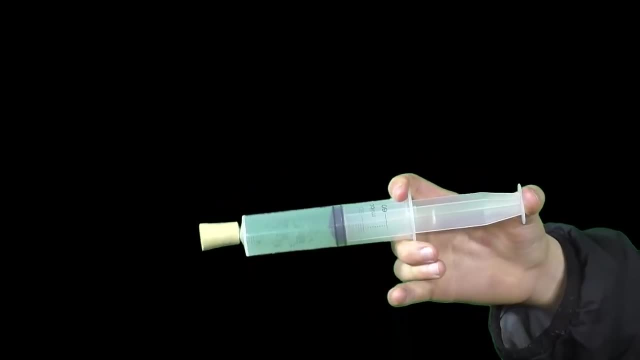 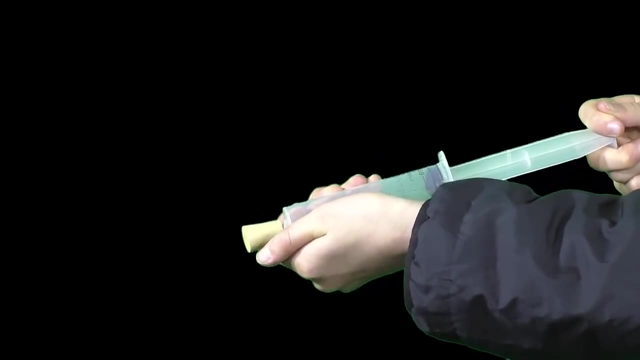 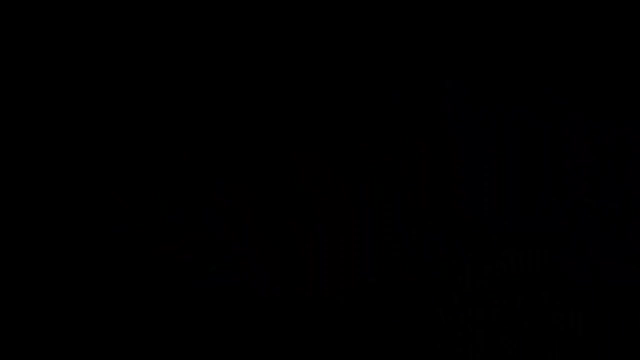 When we push on the plunger, we can squeeze it into a smaller volume Music. When we pull on the plunger, the volume expands. This means that a gas can both compress and expand to fill the entire container. Because they also have a changeable shape, they can flow and take the shape of the container they're in. 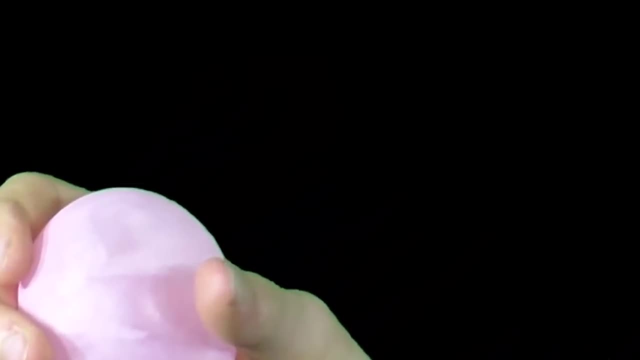 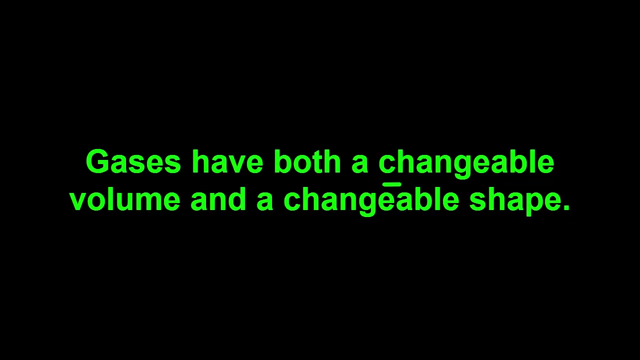 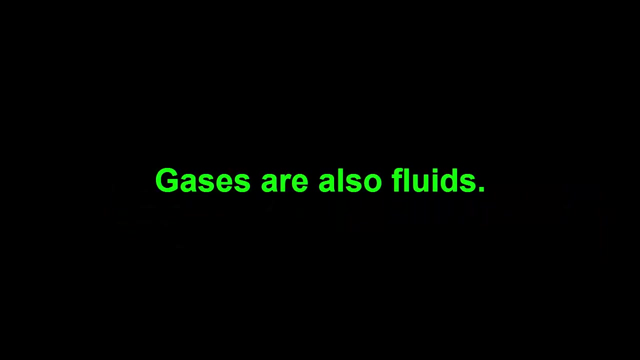 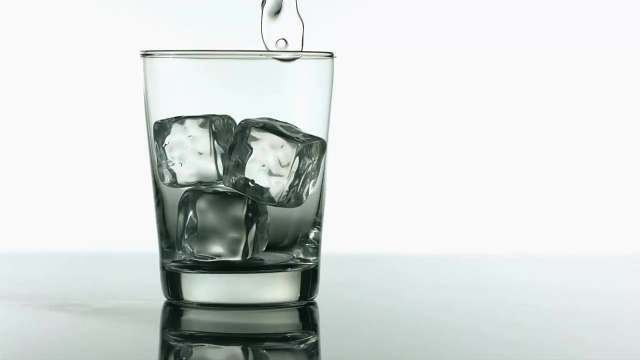 Here we're changing the shape of air inside a balloon. Easy Gases have both a changeable volume and a changeable shape. Music- Music. Because they can flow, gases are also fluids. Music. We can usually change a substance from a solid into a liquid and then into a gas by heating it up. 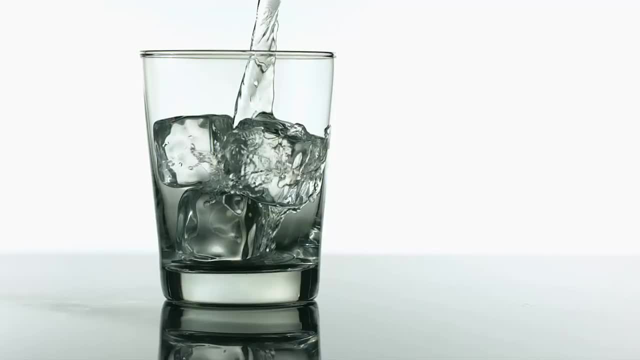 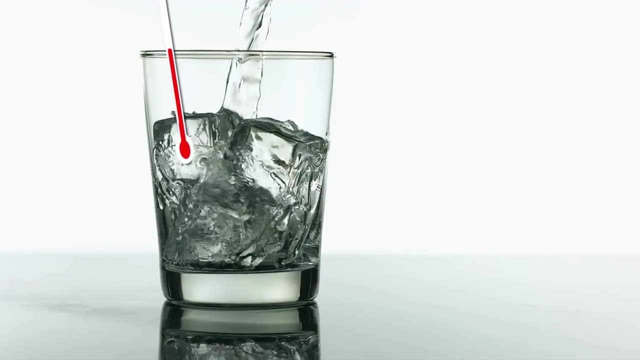 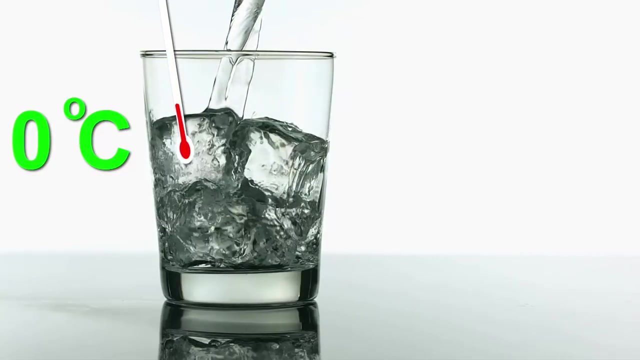 and make it go back to a liquid and then into a solid again, by cooling it down. For example, putting water into your freezer will turn it into solid ice when it cools to zero degrees Celsius Music. Once it's frozen, the ice will get even colder and might get down to minus 20 degrees Celsius inside your freezer. 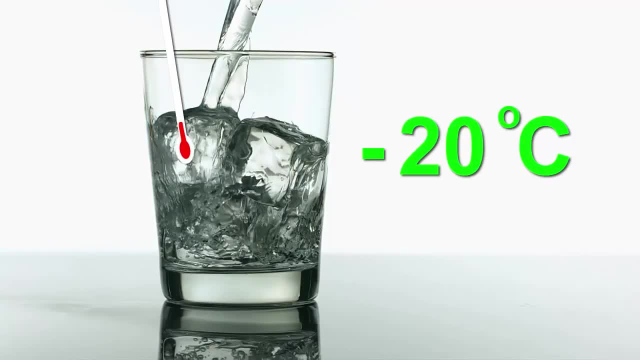 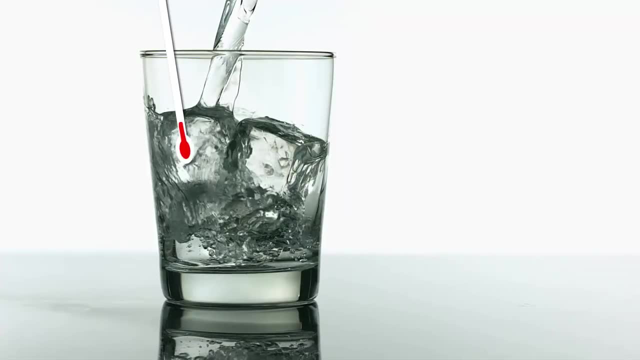 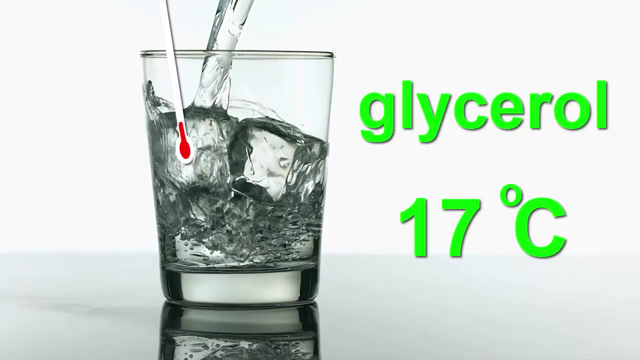 That's 20 degrees below zero. Music And different substances freeze at different temperatures. For example, we only have to cool a substance called glycerin. This means it might be a liquid during the day, when it's hot, and a solid at night, when it's cold. 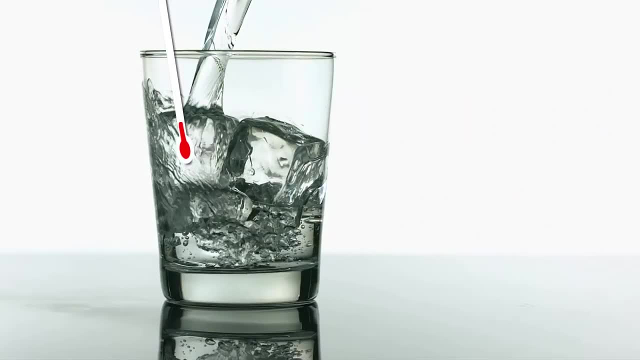 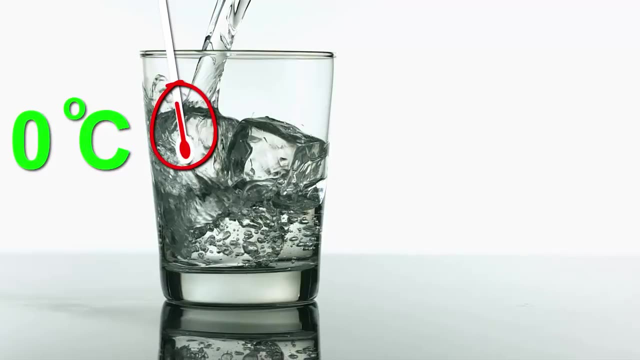 If you warm the ice, it'll melt back into water at zero degrees Celsius. Notice how the temperature that water freezes and then melts again are the same temperature. Your tap water at home is typically about 20 degrees Celsius. Notice how the temperature that water freezes and then melts again are the same temperature. 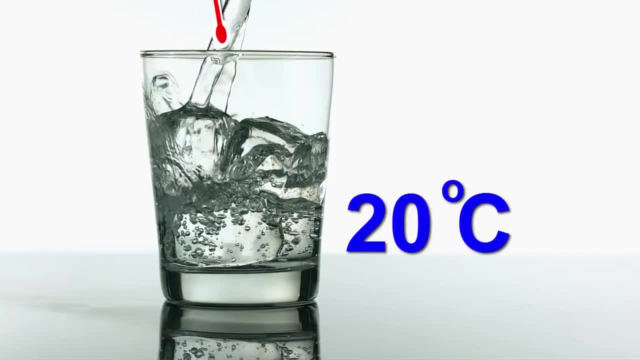 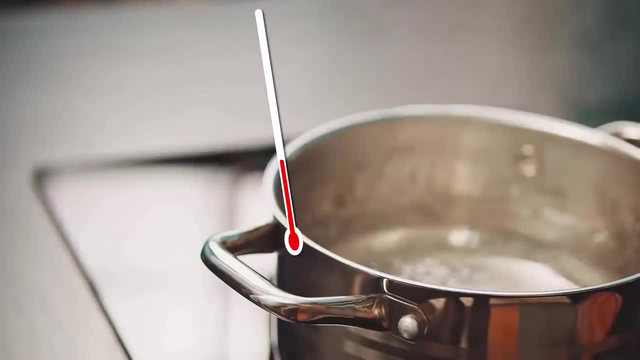 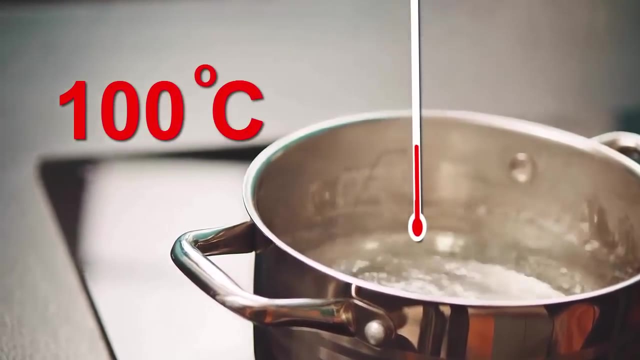 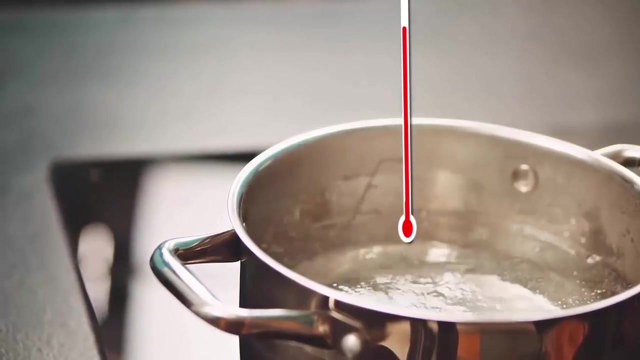 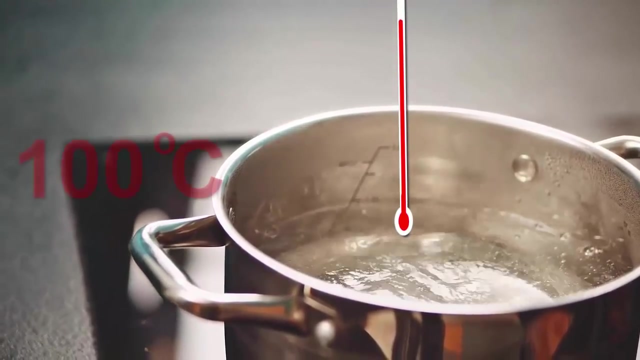 Your tap water at home is typically about 20 degrees Celsius Music. Heating it to 100 degrees Celsius will make it boil into gaseous steam Music Again. different substances boil at different temperatures. If we cool steam down it will turn back into liquid water again at 100 degrees Celsius.